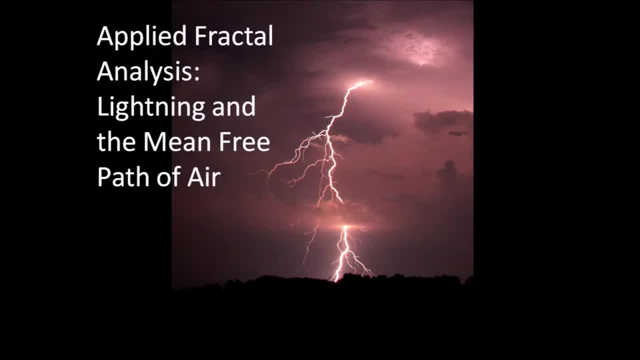 in the previous videos. The intention of this video is to show just how powerful fractal analysis is. In fact, we won't even need the full theory to compute interesting properties, So no measure theory or calculus required. Okay, so how long is a typical lightning bolt? As we've been discussing, that's kind of an 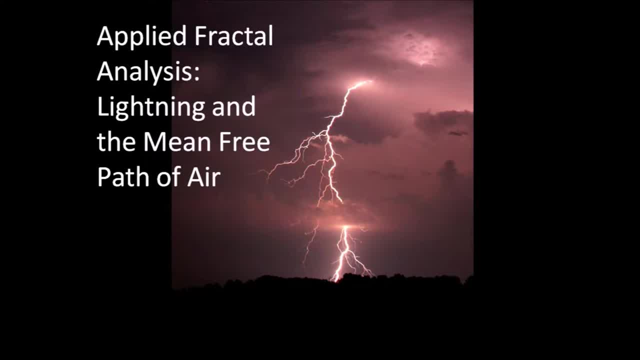 ill-posed question. The real question is: how long is a lightning bolt if the measuring apparatus measures down to a certain length scale? It's a bit pedantic, but it is completely necessary to really answer the question. So you can measure the length of a lightning bolt by measuring the length of a lightning. 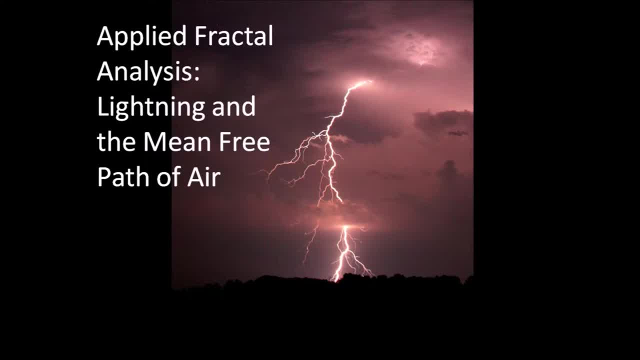 bolt. You could start by looking at the global length scale. That's the length from the cloud cover to the ground And it measures basically the linear length. But really we have other parts of the bolt that are kind of more intricate than just measuring from point A to point. 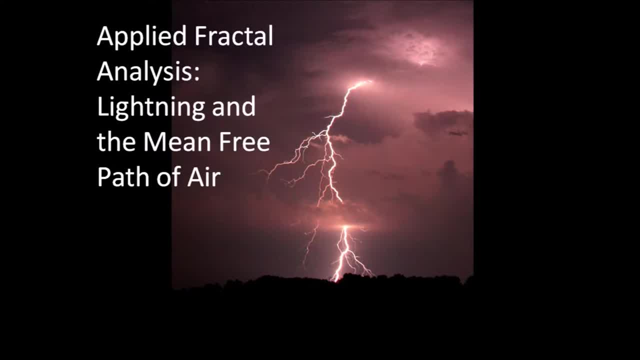 B. These points are more intricate, complex and they're actually a fractal because the length is effectively infinite. Okay, so what's the actual length of a lightning bolt? Remember, theihi is the shortest path connecting the cloud cover to the ground, but you actually have to go through the lightning. 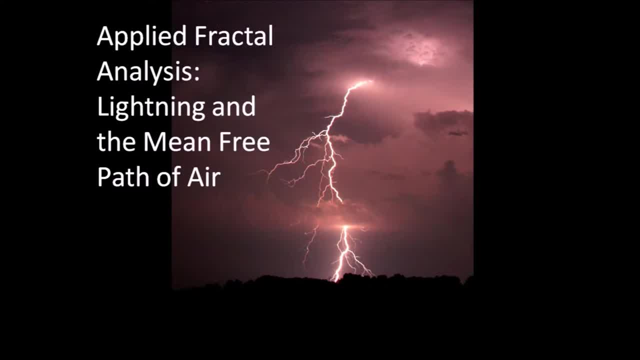 bolt. Other parts of the bolt matter, But one can argue that these fringe bolts die out in such a way that their length is inconsequential with respect to the main bolt. I am actually hoping to do a video where I discuss this in more depth, but for right now we can understand. 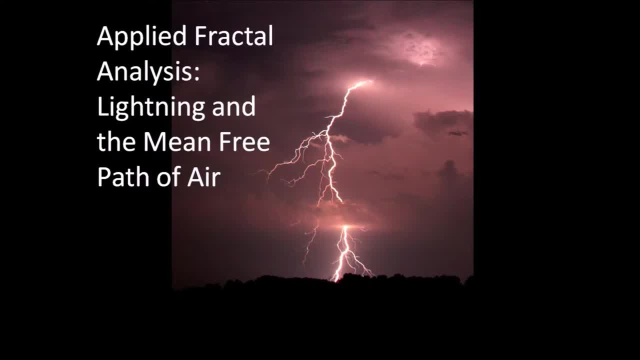 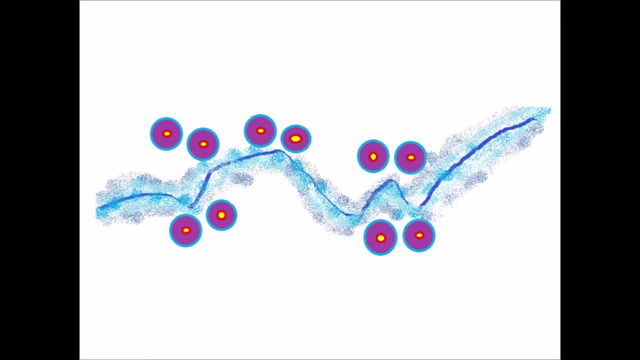 this as a removal of all parts of the bolt with fractal dimension or length scale less than the main bolt. Okay, so what's happening at the microscopic level? So I provided an amateur diagram and at this scale we have electrons individually interacting. 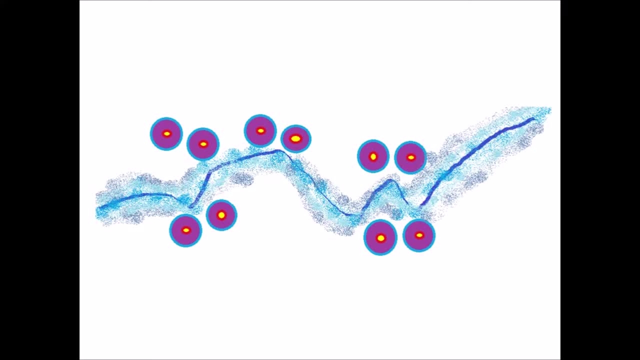 with molecules of air. So since most air is composed of nitrogen, I've only really drawn the nitrogen diatomic structures, and so we have the electron moving in a linear fashion until it gets really close to these atoms. And when it does get close to an atom, the probability that a photon will be exchanged. 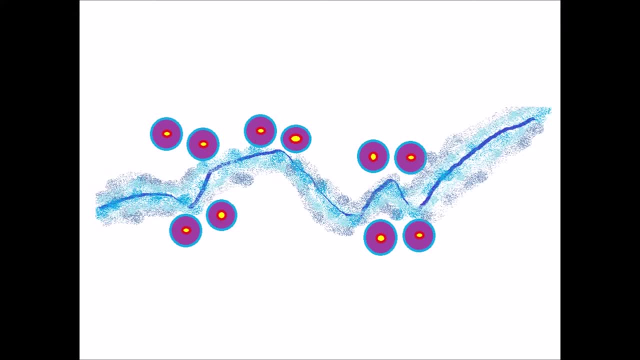 with the atom increases. When a photon is finally exchanged, the nitrogen atom's energy level is raised and the electron is repulsed away from the atom. This happens all in the span of less than a second, hundreds of millions of times. 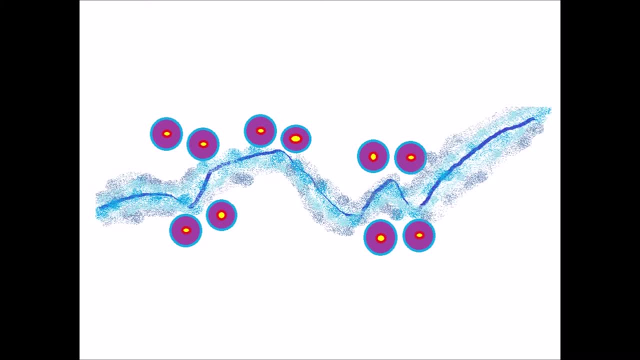 Since we have so many interactions, it makes sense to talk about the average distance between photon exchanges. This quantity is referred to as the mean free path. This scale is fundamentally important to our investigation. Below this scale, the motion of the electron is linear in a probabilistic sense, and above 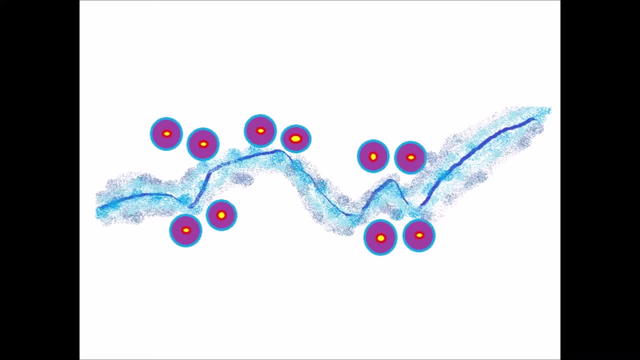 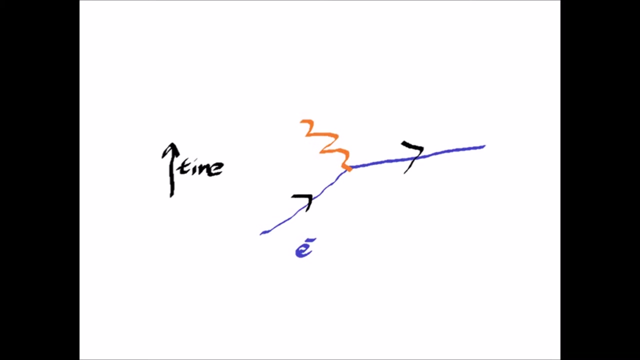 this scale, the path is highly nonlinear and fractal. Essentially, this is the scale at which fractal analysis breaks down and quantum electrodynamics is needed to properly describe the electron. So here's the Feynman diagram for what's being described with a rough semi-classical diagram. 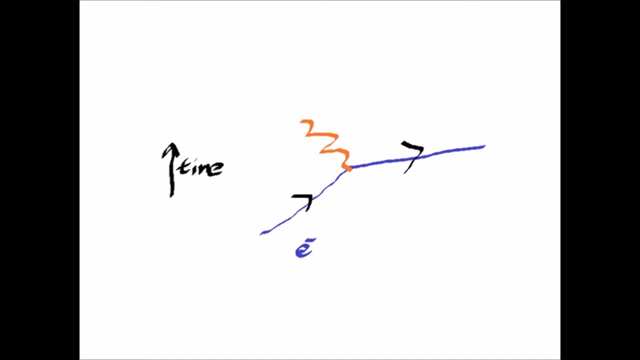 Essentially, each line corresponds to a factor that goes into an integral. Computing the integral gives you a probability for the diagram. This is the probability that this event transpires. After summing over every possible way, this event could happen, the statistical description is complete. 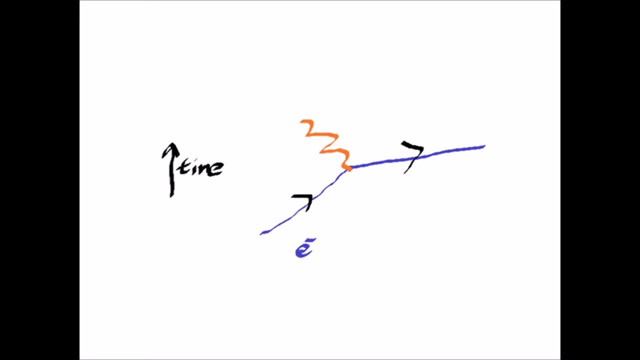 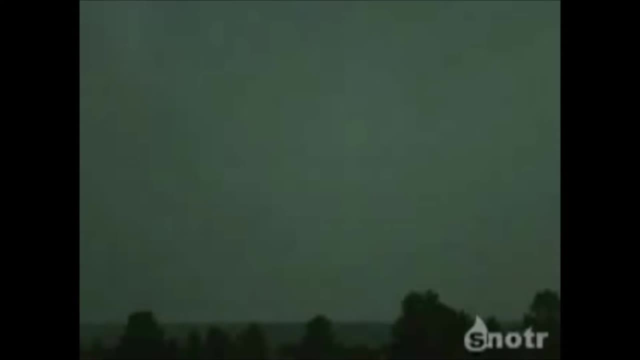 This really isn't necessary here, unless you want a Nobel Prize or something. so we're just going to move on. Here is a video of the lightning, so you can see what's actually happening here. It's traveling and it's taking the path of least resistance. Basically, You can see that it's basically having all these tendrils go down, and once we find one that has the least path of resistance, once it hits the ground you get a big flash, because all the electrons then are attracted along the path of least resistance. 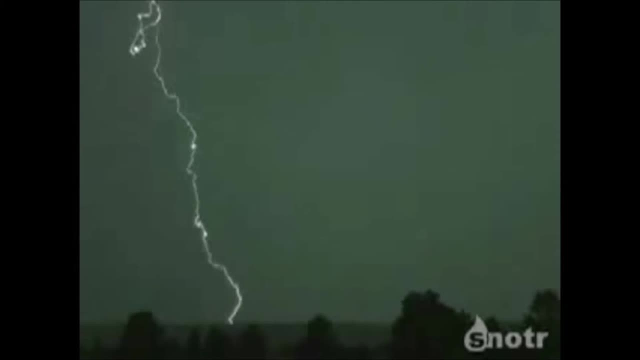 And you can once again see that all of these other tendrils go away and you're left with one mean bolt. Okay, So we have a pretty good qualitative understanding of lightning. We have a pretty good qualitative understanding of lightning And we have a pretty good qualitative understanding of lightning. 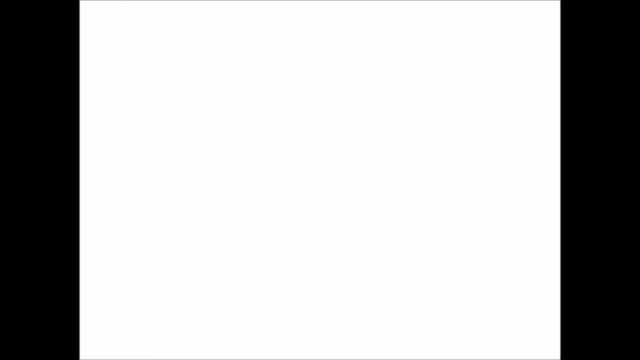 And we have a pretty good qualitative understanding of what's happening. It's time to throw some math at it so we can pull numbers out of our model. So first recall the notion of length and area. If you try and cover a unit box with smaller boxes of a half unit length, it takes four. 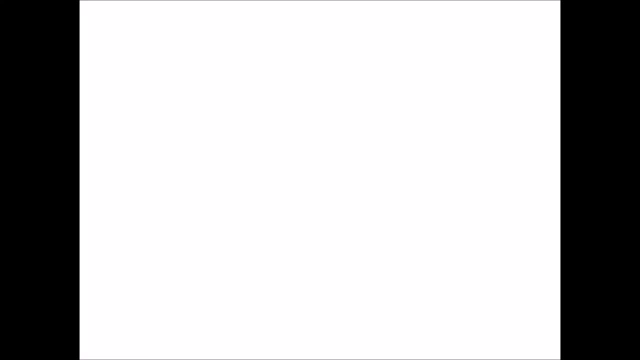 boxes to do so. However, if you want to cover a unit line with half length unit lines, it only takes two. This is described by the above formula. D is the global length of the line or box or, in our case, lightning bolt. 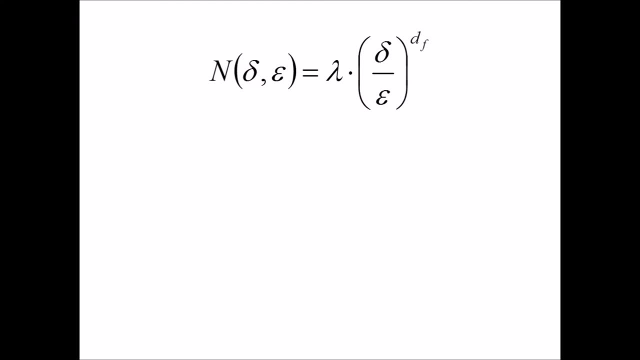 Epsilon is the length scale of our covering line or box For lightning. this length will be the mean free path. Okay, And d is the dimensionality of our object. For a line, this number is one. For a box, the number is two. 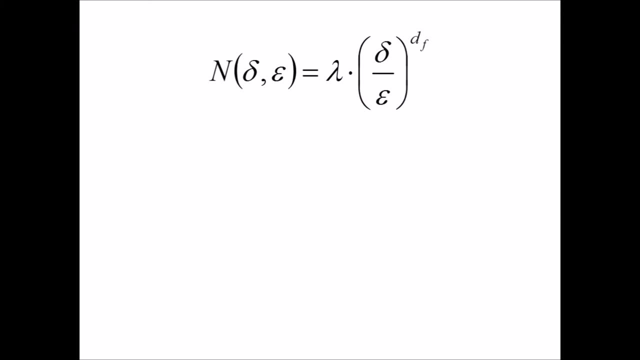 However, for lightning, this number will be some number between one and two. Now, Each covering box we use contains part of our object. Since we want the length of our bolt, we have to multiply each box by the length of the lightning contained in it. 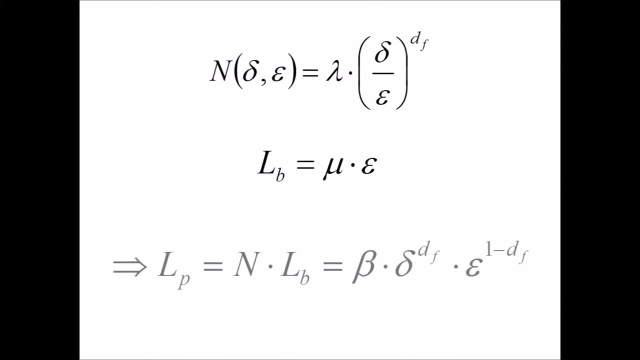 This amount will be proportional to epsilon. Putting this all together, we obtain an equation for the length of a lightning bolt measured at some scale- epsilon. Okay, So let's quickly discuss the various scales involved in our model. The first is the length of the bolt at the minimum scale, epsilon. 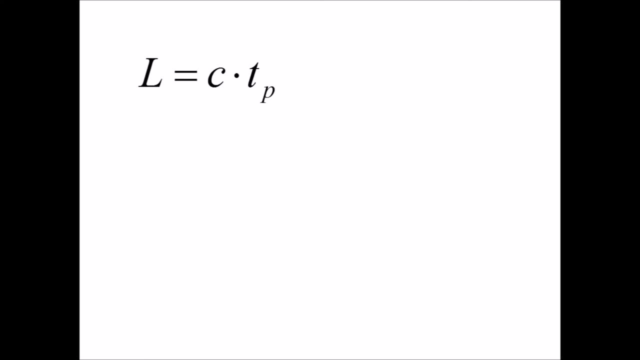 Assuming that the length of the bolt is equal to the length of the bolt at the minimum scale, assuming the electrons are traveling near this speed of light, we see that it takes some amount of time- t of p- for the bolt to travel from the clouds to the ground. 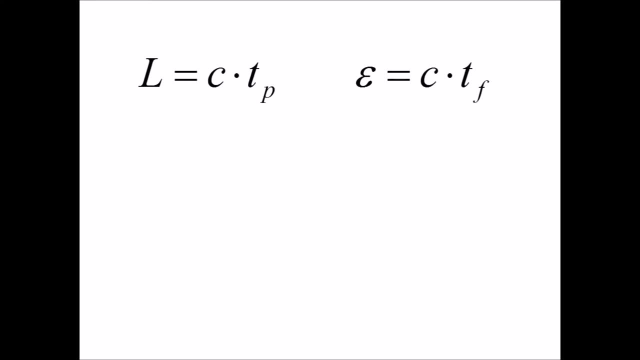 The next scale is epsilon, the mean free path. So it takes some amount of time- t of f- for the electron to cover this amount of distance. This is also the amount of time an electron travels undisturbed by the surrounding air particles. 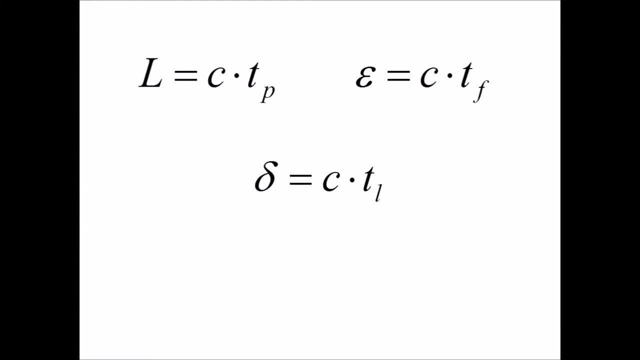 The final length scale is delta. This is the direct linear distance from the clouds to the ground. This is the length of the bolt at the minimum scale, epsilon. The time t of l in this case denotes the amount of time an electron would take to travel. 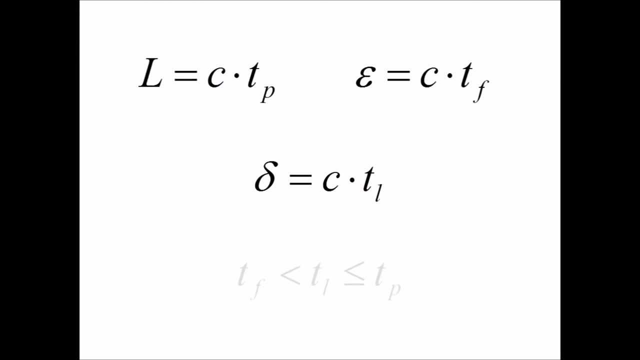 this distance if it was completely unperturbed. We can then order the relevant time scales in order of their size. So we have t of f less than t of l less than t of p. Okay, So now that we've set everything up, let's actually solve for the amount of time an electron 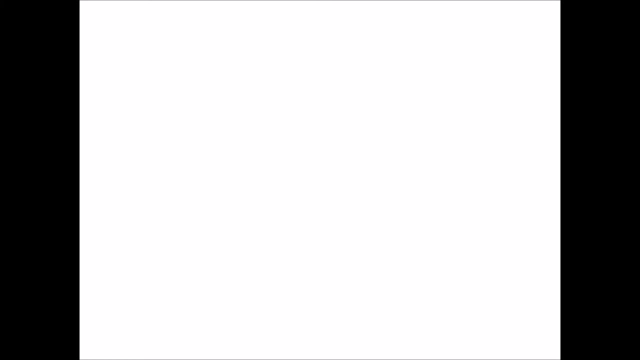 travels unperturbed, since it's basically the only question about lightning that we can't directly see from photographs. So we can do this by substituting our time relations into the length equation we previously derived. It's pretty much algebra at that point. 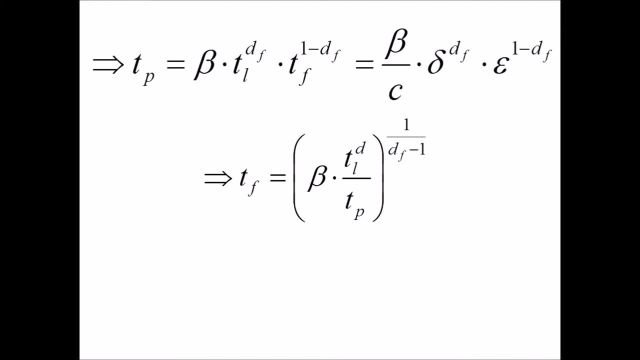 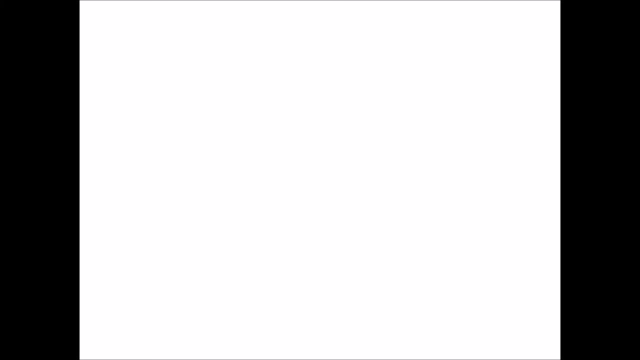 an electron. So here are our two important equations for the mean free path, and we also have an equation for the total propagation time of the electron. Okay, So let's put in the values that are relevant for us so we can get some numbers out of. 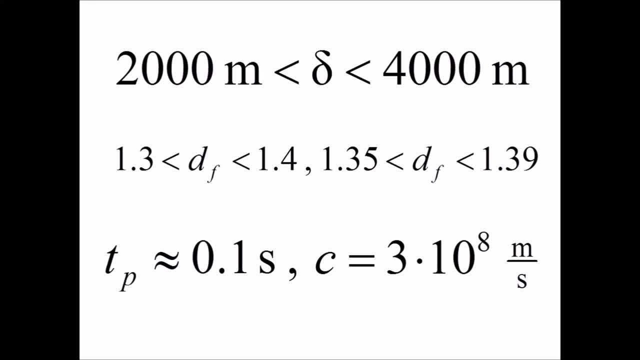 our equations. Most of these are pretty easy to find online. let's see, for instance, we have a 2,000 meters to 4,000 meters- that's about the average height of cloud cover- and then we also have the fractal dimension, which 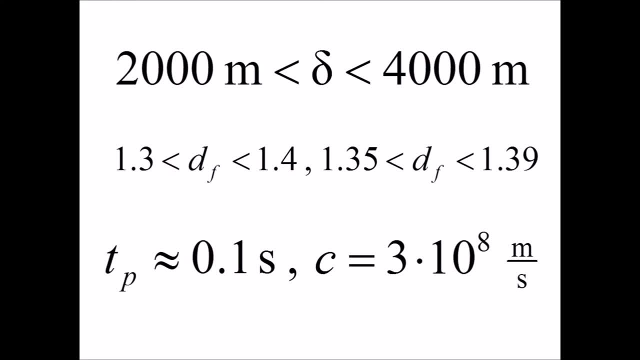 is actually completely estimated by the photo provided in the first clip, and that's 1.3 to 1.4. and then we also have a theoretical prediction of 1.35 to 1.39. we're gonna actually use both. and then we have the propagation time of the. 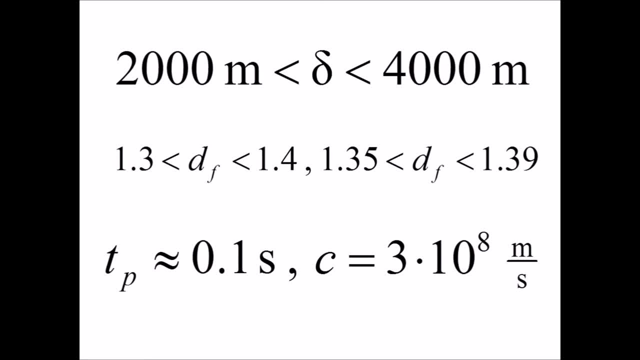 video I showed, which is about a tenth of a second. now, to get that value, I just looked at the frames per second provided in the video, which is about 7,000 frames per second, and then I took the 60 frames per second. that corresponds to the real. 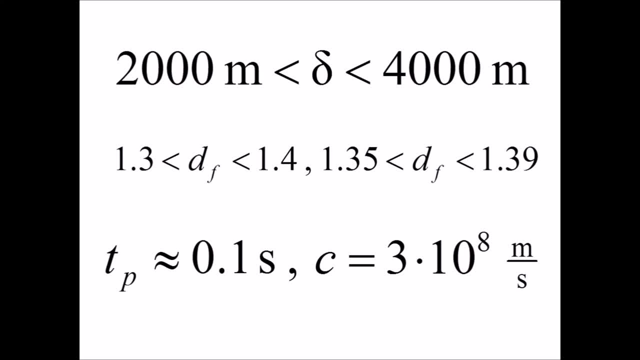 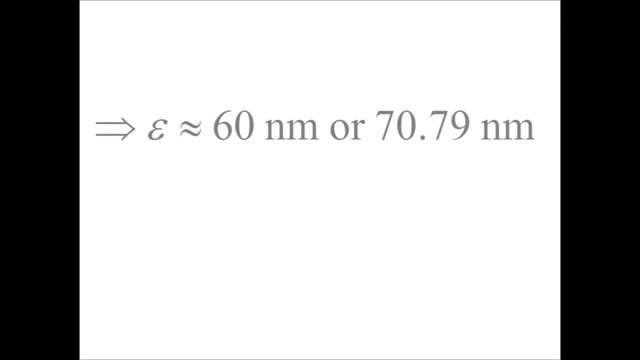 world, and then I just divided those out, and so that's how I got 0.1 seconds, okay, and then we finally have the speed of light, which is going to be very relevant to our calculations. ok, so using these values, we get that. the mean free path is about 60 nanometers, or. 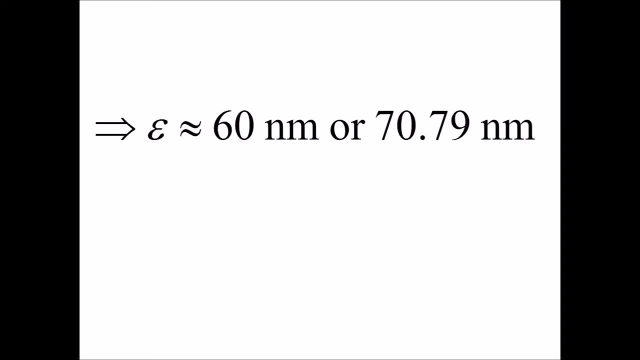 70.79 nanometers. if you use the more specific value for the fractal dimension. this should be compared to the values given on Wolfram for the mean free path of air. ok, so if we use these values for the mean free path, then we can actually also derive. 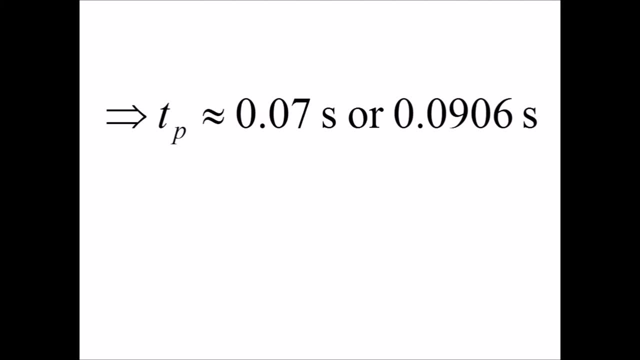 the propagation time and doing this, we get about 0.07 seconds or 0.09 seconds respectively for each fractal dimension estimate. now, that's actually pretty close to the 0.1 seconds that we saw in the video, and I did use a bit of a weird method to get that, so really either. 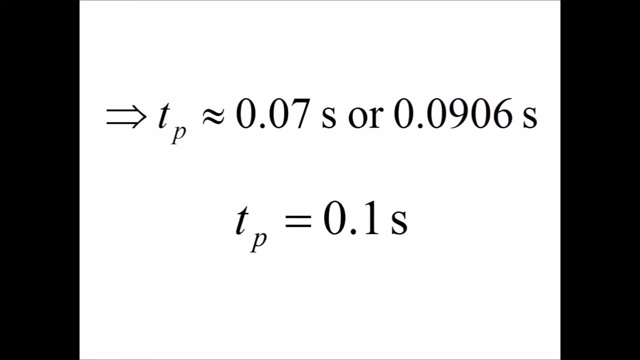 of these values could really be considered the true value. ok, so finally, if you are willing to work a bit, you can derive the total energy in a typical bolt of lightning. so, since we have the mean free path, we know that the number of interactions along the electrons path is equal to the travel length divided by the mean path. we also know that 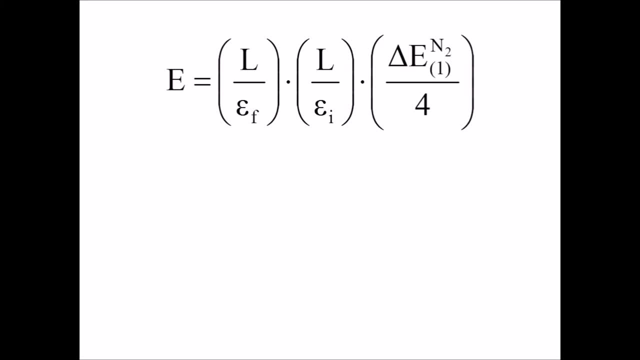 each of the electrons interactions is uh causing energy to be radiated in the form of protons. at this level, quantum uh interactions uh are very important. finally, uh, since I have no interest in doing a uh full quantum electrodynamics calculation, we'll just assume that an average interaction with a photon 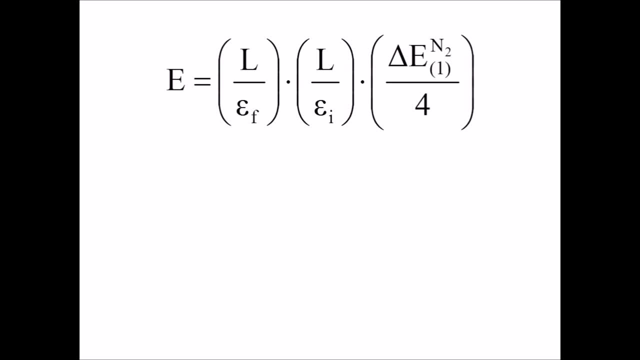 causes the energy of the nitrogen to rise one fourth of a energy level. now, once the first several electrons have carved out the path of least resistance, the others are going to follow the same path. so we multiply by the length of travel divided by the mean free path, however, the air temperature will be much, much hotter. 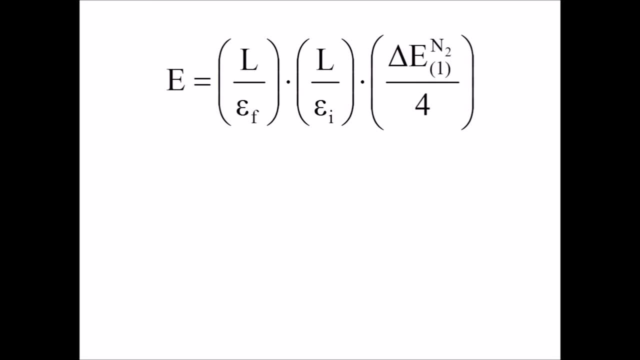 in fact it'll be about 30,000 celsius or 53,000 fahrenheit. this means that the mean free path will increase, so collecting up all the values that will be relevant is a bit of a chore, but it's not very difficult, uh, if you just use, uh, wikipedia and wolfram, I'll actually 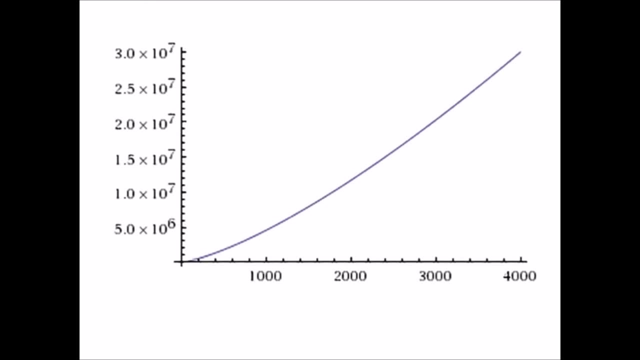 provide some links in the uh description. so if you put everything together, you will get about 1.1 billion joules for the energy. okay, so that's enough power to power a home for a month, melt a ton of steel or run an experiment at CERN. okay, so we've been seeing.